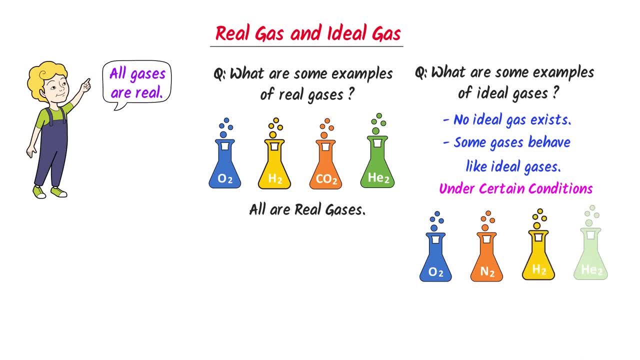 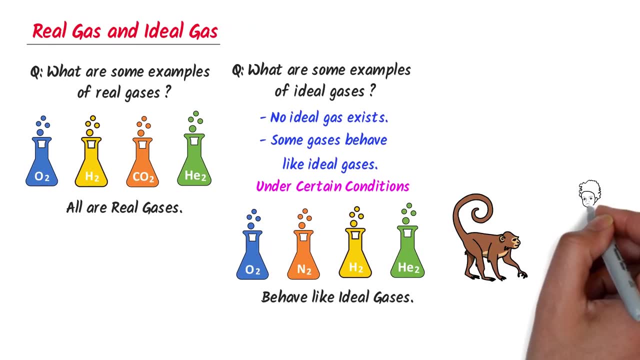 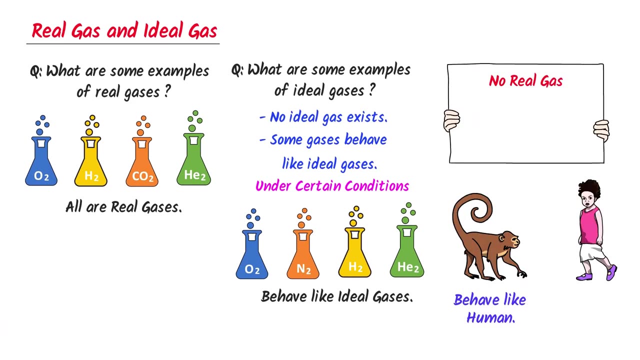 gas, nitrogen gas, hydrogen gas and helium gas behave like ideal gases. For instance, chimpanzee is not a human being, but any chimpanzee can behave like a human being. Similarly, no real gas is an ideal gas, but some real gases behave like ideal gases. 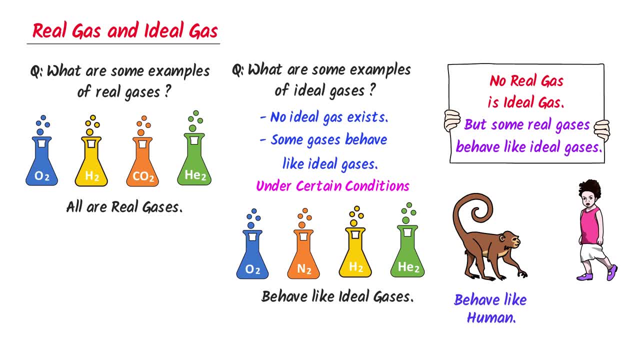 Thus we have learned two important concepts in this slide. Firstly, all gases in the universe are real gases which we use in our daily life. Secondly, some real gases can also behave like ideal gases under certain conditions. Hence, note it down, all these important points. 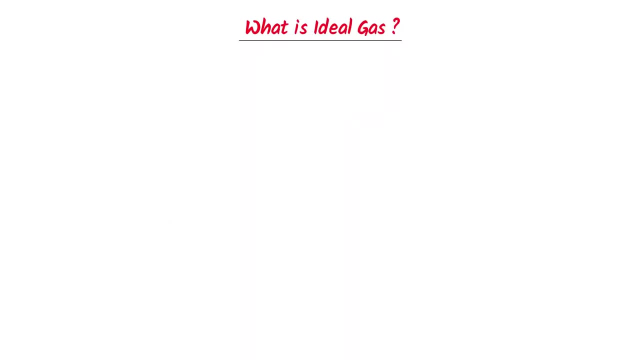 Now, what is ideal gas? Well, consider hydrogen gas. We know that it is a real gas. Now I am interested that hydrogen gas should behave like ideal gas, So I have to change certain conditions for it. For instance, we know that gaseous behavior is affected by the pressure and temperature. 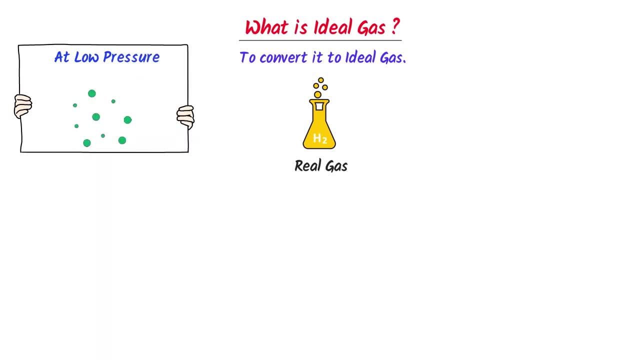 For example, at low pressure, molecules of hydrogen gas behave like ideal gases. So hydrogen gas abandons theила when heat is wielded. So now we know that своим energy is enjoyed when high pressure becomes low. Let's to that Grill and we will use that. 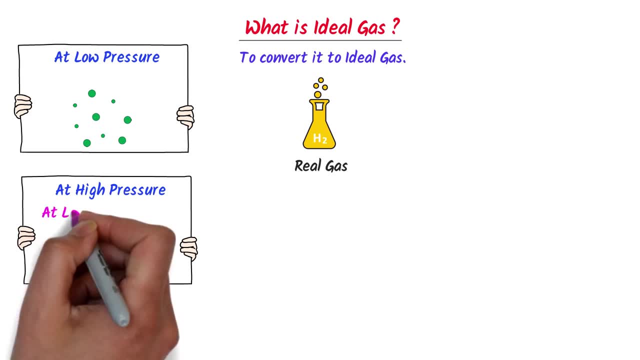 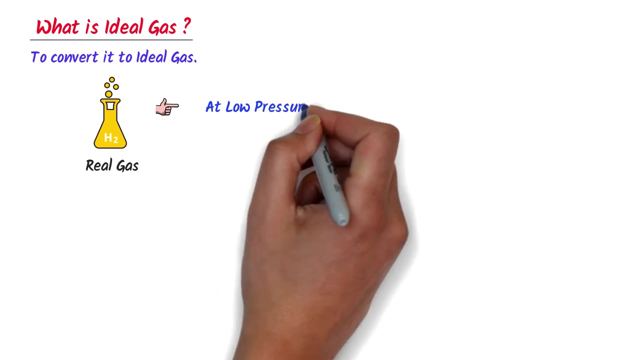 now, Before I continue on from the next video, I would like to mention one more important fact. When you enter into the Bl, prettiest region of the universe, the every halve of the universe contains only three sides. What is Im interpretation? 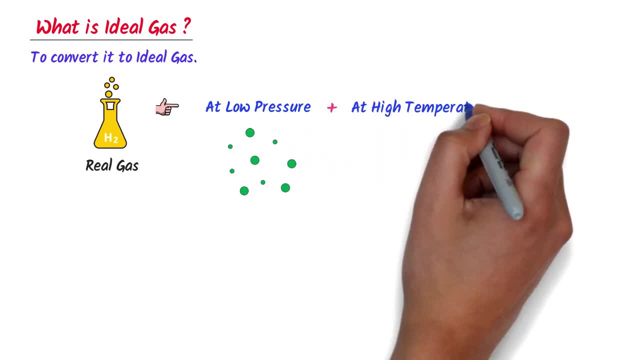 It is simply two channels. The right above is fungal In the signal, known as nurses followers' channels. The left above is medial. The top is mulheres provide very high temperature to it. As a result of this, the molecules would further move away. 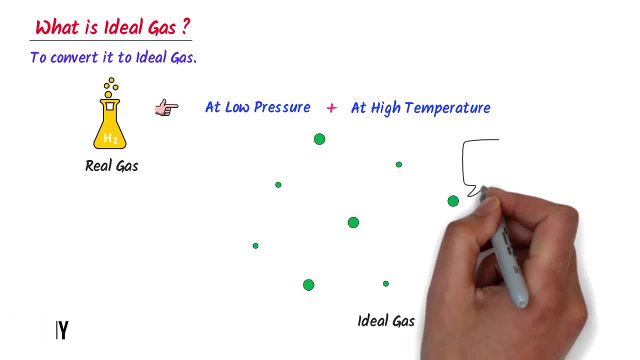 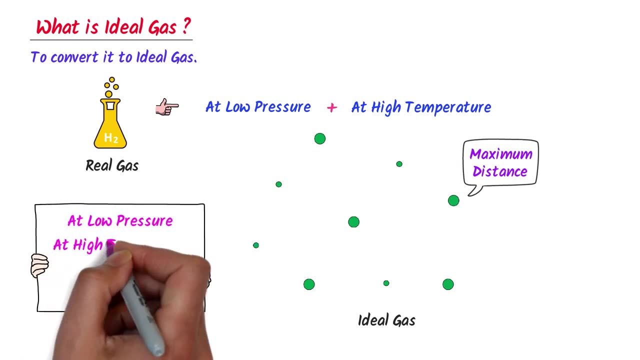 from each other, So we can see that molecules are at maximum distance from each other. Thus we say that at low pressure and high temperature, hydrogen gas behave like ideal gas. Let me repeat it: At low pressure and high temperature, hydrogen gas behave like ideal gas. Therefore, remember that. 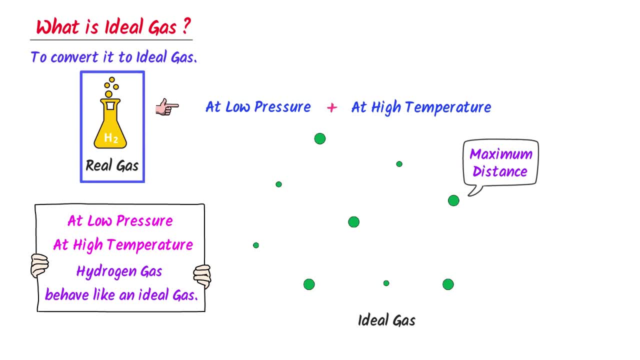 this hydrogen gas is a real gas which we use in our daily life, While this hydrogen gas at low pressure and high temperature is behaving like an ideal gas. Thus we learn that at low pressure and high temperature, some real gases like hydrogen gas can behave like ideal gas. 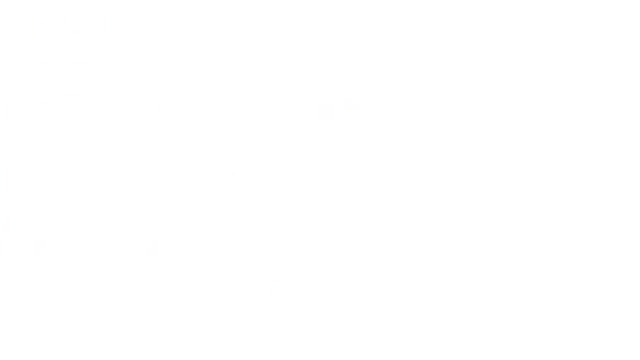 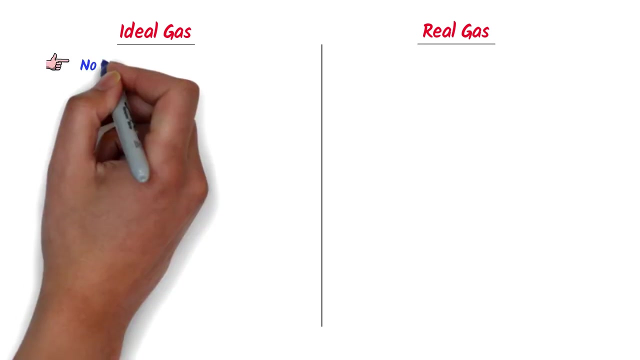 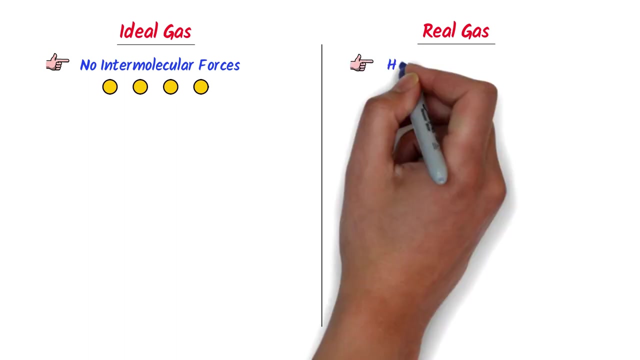 So this is the whole concept of ideal gas. Now, what is the difference between ideal gas and real gas? Well, in ideal gas, no intermolecular forces of attraction exist between molecules, While in real gas, intermolecular forces of attraction exist between molecules. Secondly, 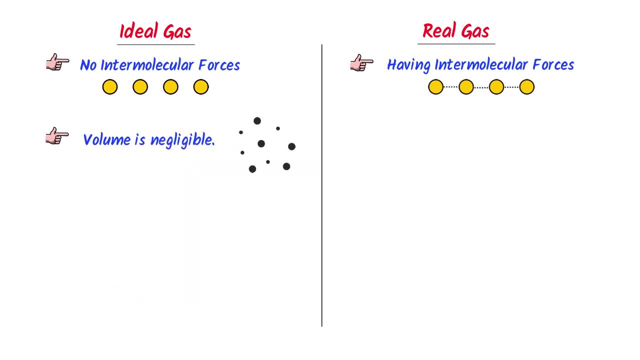 in ideal gas the volume of gas is negligible. It means that the gas is at low pressure and high temperature. Thus we can say that at low pressure and high temperature gas is not taking up any space, While in real gas the gas molecules take up some. 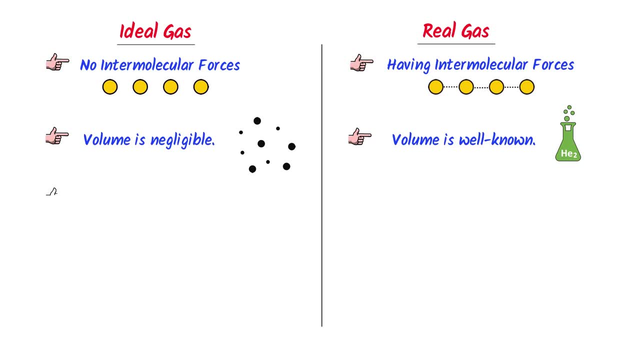 volume in the container. Thirdly, in ideal gas the collision between gas molecules is perfectly elastic collision. It means that when gas molecules collide with each other, no energy is lost. While in real gas the collision between gas molecules is non-elastic. It means that when gas 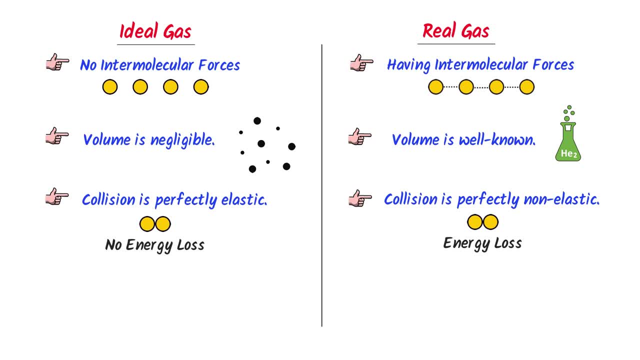 molecules collide with each other, no energy is lost. Fourthly, in ideal gas, the gas molecules follow the ideal gas equation, PV is equal to nRT, While in real gas, the gas molecules do not follow the ideal gas equation, PV is equal to nRT. Thus, these are the main differences between the real 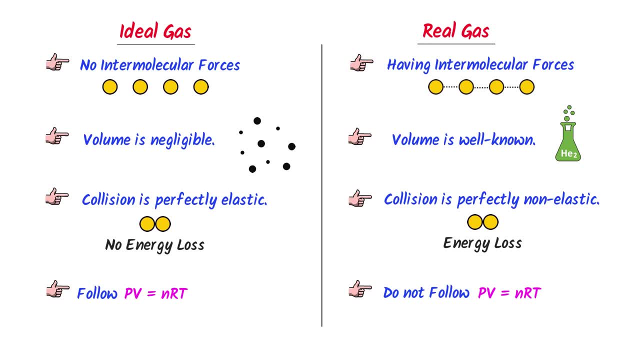 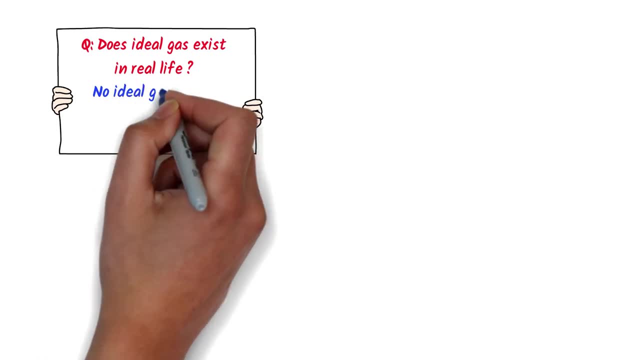 gas and the ideal gas. Finally, let me teach you three examples of ideal gas. First of all, the exam questions: Does ideal gas exist in real life? The answer is no, No ideal gas exists in our daily life, But many gases, like hydrogen gas, behave like ideal gas under certain conditions. 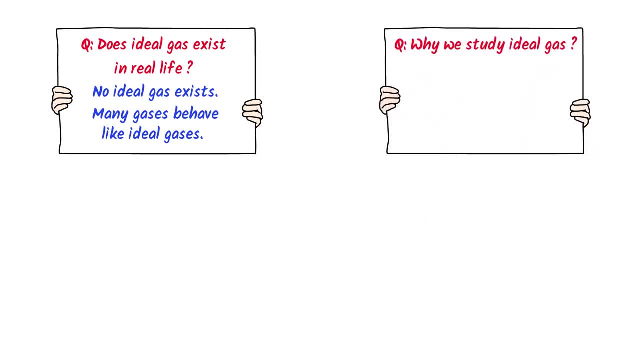 Secondly why we study ideal gas. The answer is simple. This concept is very useful because, using this concept, we can easily learn and understand the behavior of any gas. Secondly, using this concept, we can easily calculate the property of any gas.